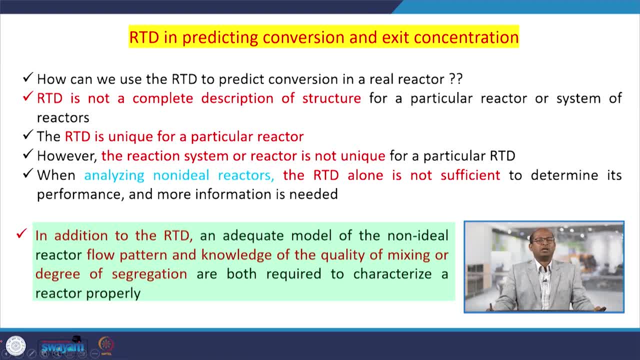 systems or reactors is not unique for that particular RTD. So for a particular reactors, whatever we have designed that particular reactors, we have to measure a particular RTD. based on that we can find out the concentration and exit concentrations, conversions, that we can find out. So in addition to the means, RTD or residence, 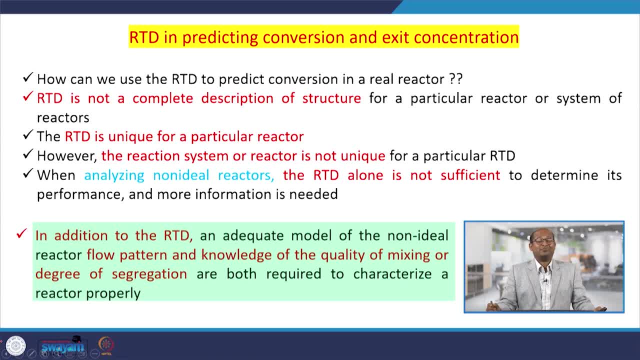 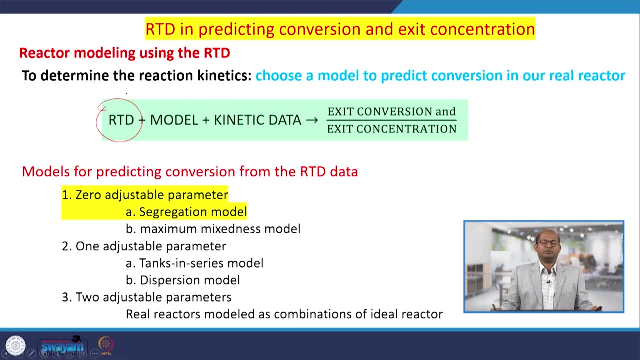 time distribution function, So flow patterns of that fluid that is feeding from the reactors. So that quality of mixing means that we should know, or the degree of segregations. So therefore, with the RTD models or for any reactors, you, once we know the RTD, or residence time distribution. 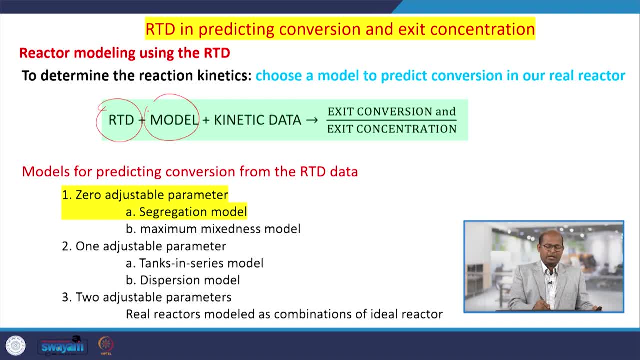 functions with that. we have to develop some models and kinetic data that we needs So once we know then exit concentrations and exit conversions that we can find out for that particular reactor. So there are so many models are available for the residence time distribution functions to predict the concentration and exit conversions for that. 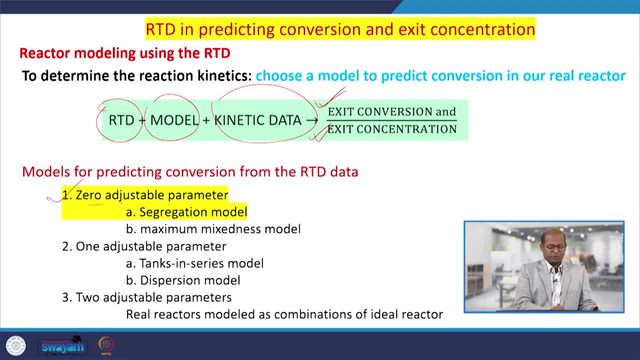 particular system. So 0 adjustable parameter models, that is called segregation models, MF models, 1 adjustable parameter model, that is the 10 series model, dispersion models, and two adjustable parameter models, that is the real reactors models as combinations of ideal reactors. so therefore, so first we will discuss about the 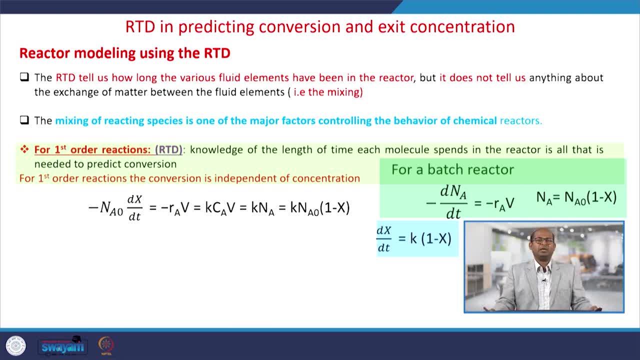 segregations model. so in the segregations models it actually tell us about the mixings of the materials or that reactant molecules that is feeding in the reactors. so whether it is proper or not, so, or with the help of this, we can find out the or predict the conversions. 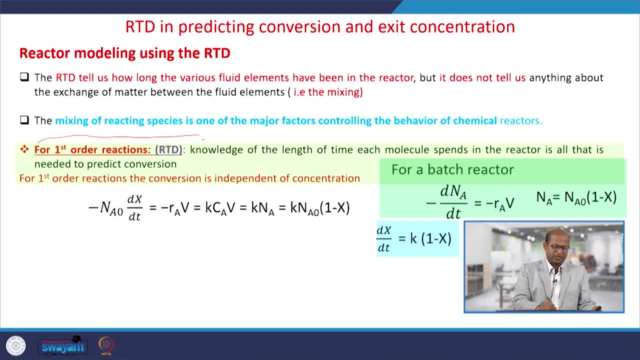 or concentrations. so for a first order, let us say for a first order reactions, if we know the design equations for the batch reactor. so let us say first order reactions we want to conduct in a batch reactor, so, and then the design equations. we can write this way: 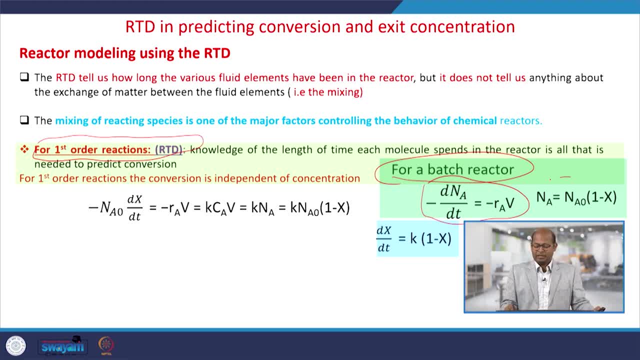 minus dNa by dt equals to minus Re into V, and Na equals to Na0 into 1 minus x, and dx by dt equals to k into 1 minus x. so here is: if we substitute this in here and then if you simplify, then we can get it this, or you can write this for a first order. 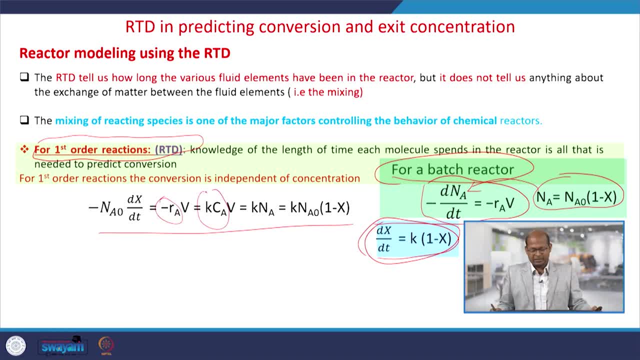 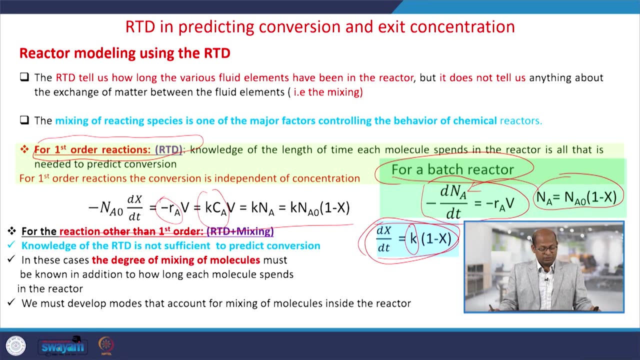 reactions. here rate we have considered first order and considering that we can get. it means changes of the conversions as a function of temperatures. so here is kinetic parameter, that is the rate constant for that particular reactions. we should know and then we can do it. so RTD and mixings, both we know. so means degree of mixing. so when that molecules are. 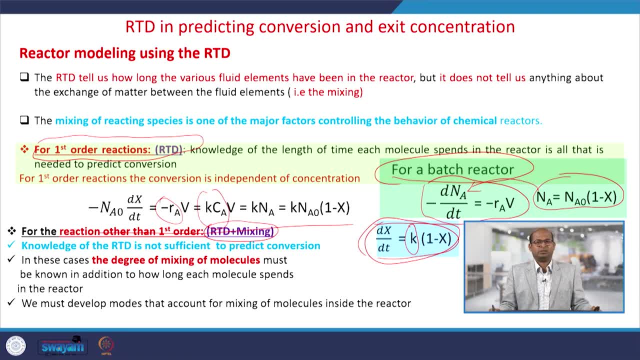 passing through the reactor. so molecules, each molecules, should pass through the reactors and that whenever it is passing through that reactor, so it may. if, let us say, two different molecules passing through the reactors, so then if two molecules come in contact and properly mixed, come in contact at particular temperature, then reactions may. possibility. 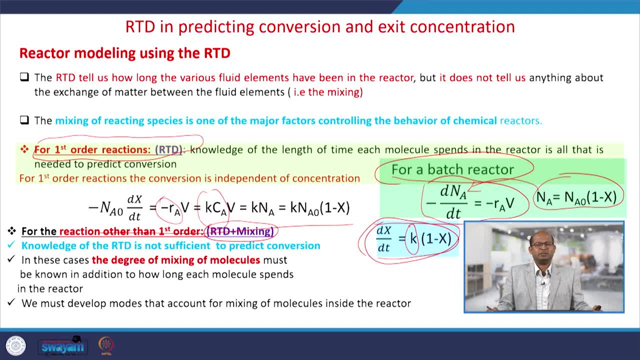 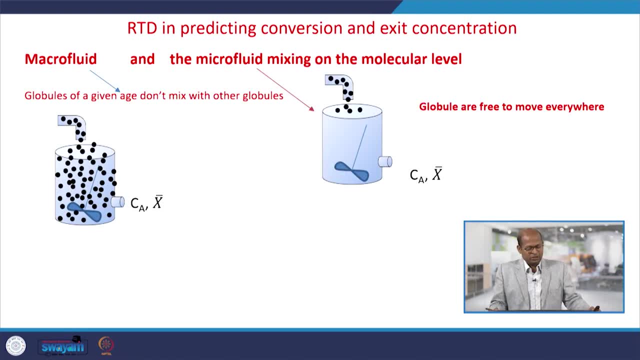 if the mixings is not proper and two molecules does not come in contact each other. so then there the means, reactions or conversions that would be different from expected. so here the mixings that we can say. it is micro fluid or macro fluid mixing, so two different way. 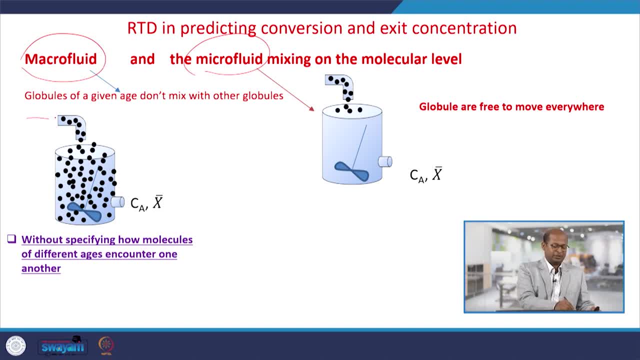 means molecular level. we can think here so when this is the entrance of a or feed inlet points of that particular reactor. this is outlet point. so here, so when molecules is entering from here to leaving this way, So we can see that the molecules in that, in the form of a spherical means we are considering, 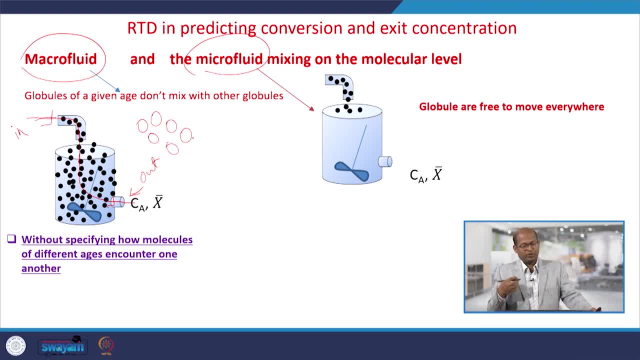 a small bubbles. so where, inside of that, molecules which presents, here also molecules which presents, but here the molecules in this globules and in this globules are different. so, but in this globules, so what are? the molecules are present, they are mixing each others and they are having. 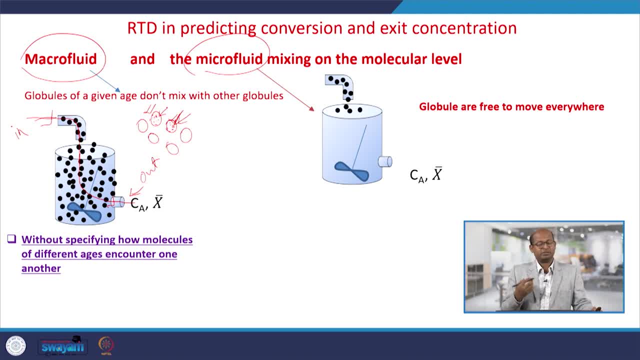 the same residence time. So in this globules having molecules, all molecules spending as same or equal times when they are passing through the reactor. but these two means molecule, these globules and these globules residence times and mixings are different. so individual globules we can. 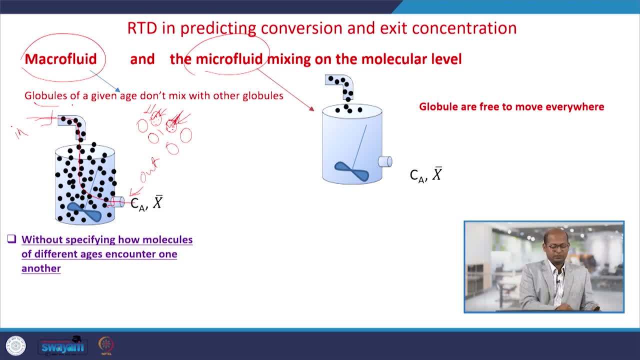 consider as a unique molecules that we can consider. So if it is does not mix these globules, does not mix with these globules, so then individual globules, So all the molecules present. they have unique residence times and unique space times for. 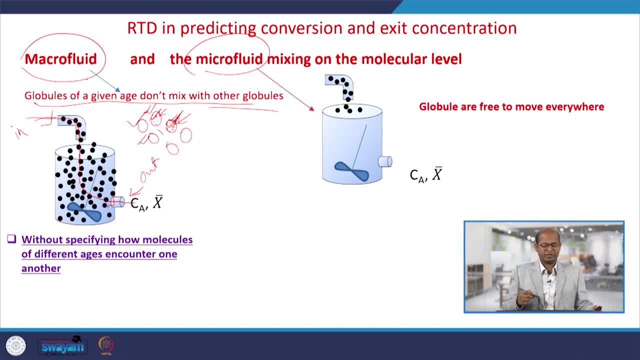 that particular reactors, and here the mixings is called microfluidic mixing, and when the globules is enter. in the second cases, here globules enters or molecules enters after that when it is mixing. so mixing the molecules is very small, means all molecules, mixings together. here mixings is called microfluidic mixing. so here mixings is proper, so all molecules. 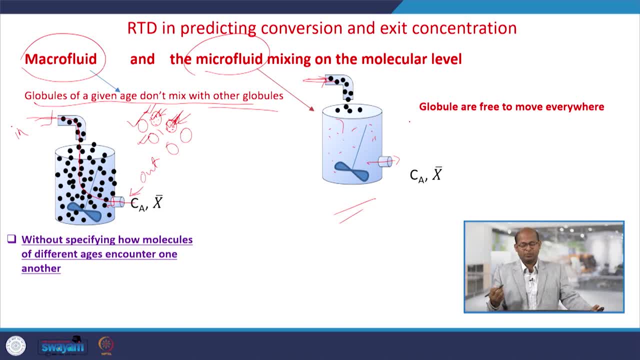 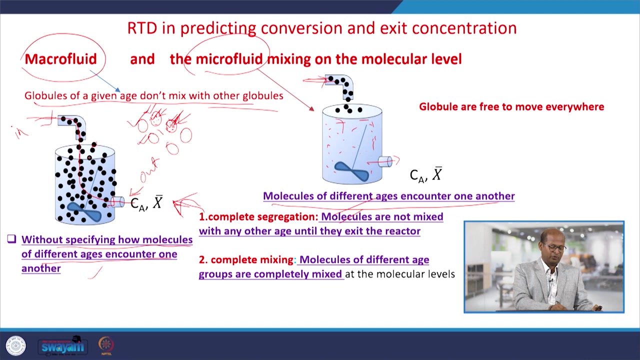 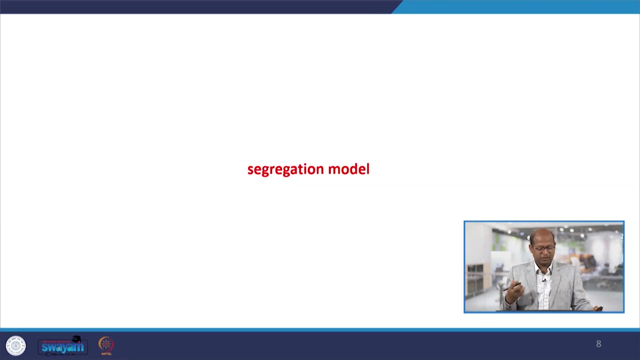 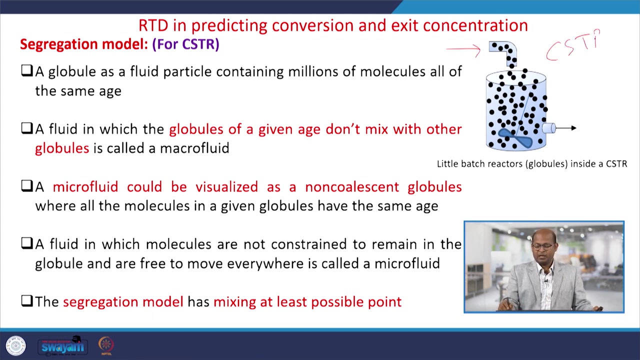 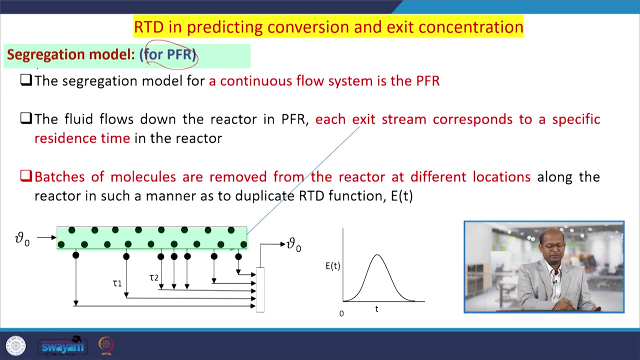 also spending The residence time, so here. so when that molecules entering inside of the reactors and then it is leaving from the reactor, so then the space time that is spent, that molecules leaving from this particular point 1 is tau 1, from point 2 it is tau 2.. 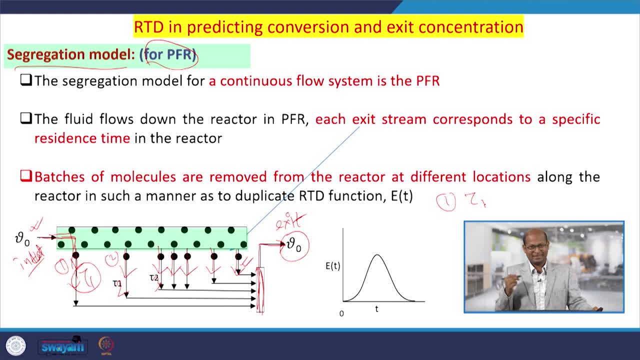 So point 1,. so the molecules spending it has the residence time or space time, that is tau 2, and at point 2, the molecules having residence times or space time. that is like this: So individual molecules having different residence times or space time. therefore each molecule, 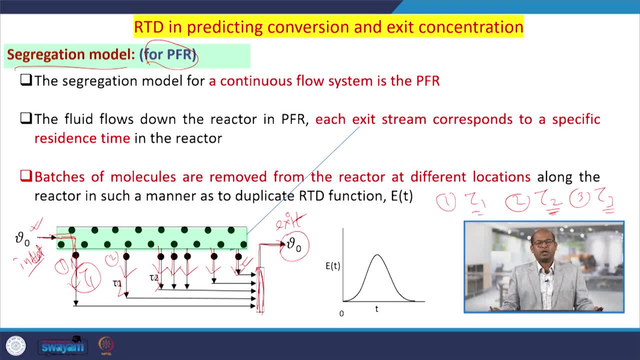 spending different time inside of the reactor for conversions. So therefore, overall, this is the model systems for PFR reactors And this is the E curves, or whatever the concentrations will come out, and based on that, if you draw the exit distribution or RTD functions for this particular system, it would be like this: 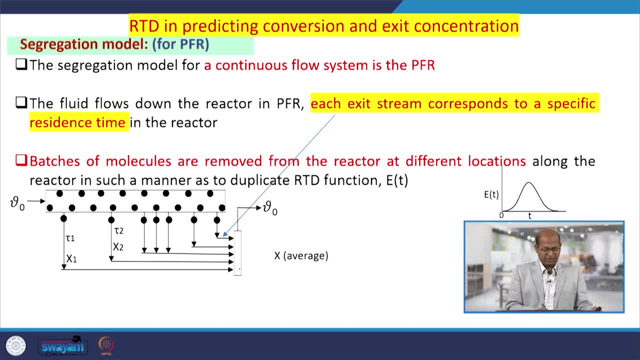 So now. so here That is the means here, if we consider at this particular point, at point 1,. so when molecules spending tau 1, space times, it has a conversions x1. and at point 2, that has space time, tau 2 and conversion is x2.. 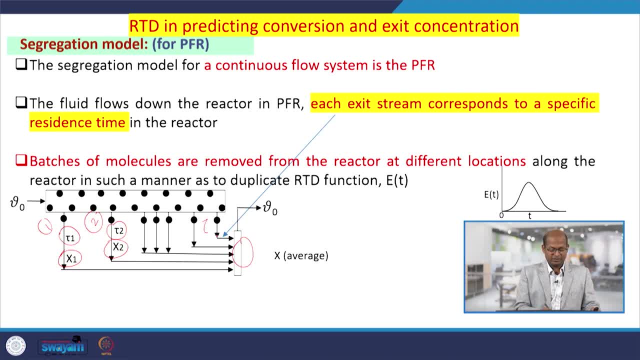 So like that, this is the exit point. so here space times and corresponding conversions here, from here, from the outlets, after mixing all point, here the conversions will get that. this is the average average conversions that will get. So if we have to sum up x1,, x2,, x3, xn point and after that if we take average, so then 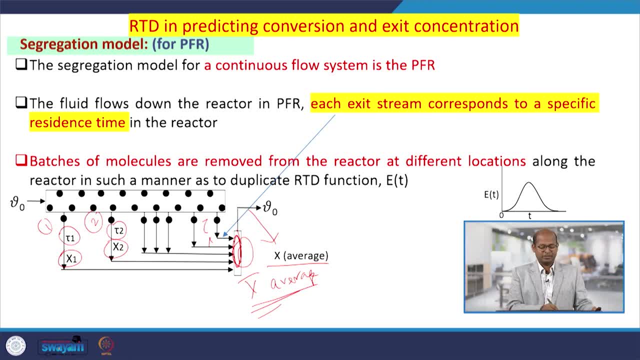 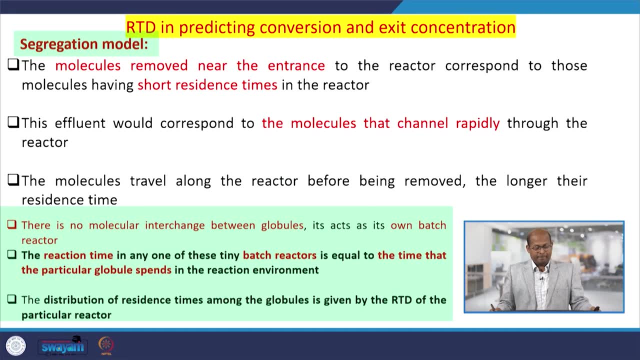 that will get average conversions for that particular system. This is the model system. So now, so now, So in this particular model, So, ah, So the molecules moved near the entrance, it has short residence times and the molecules that channels rapidly through the reactors. this corresponds to the effluents. 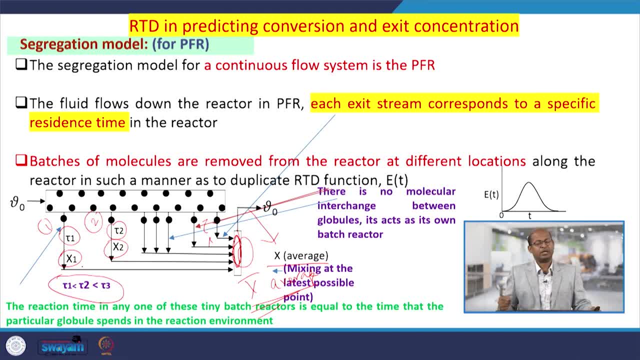 So here I said this way it would follow the residence time distribution or space times. So, at this particular points, molecules having less residence times or space time and at this particular points, molecules having longer residence times or space times that spends longer period of time. So what are the globules, or molecules or individuals globules we are considering. 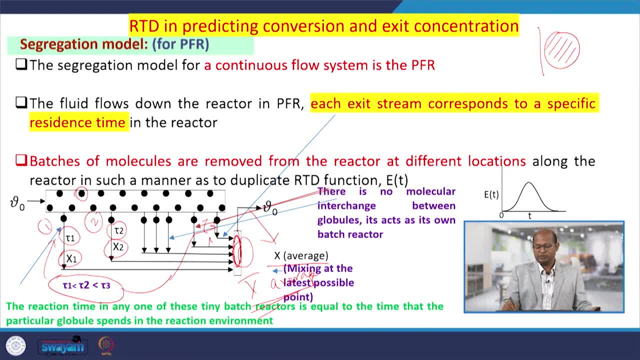 So let us say this is the globules. inside of that globules it contains molecules. what are the molecules? and inside of these globules we can say that it is as small and here, whatever the conversions is taking place, and individual globules we can consider as a batch reactors. 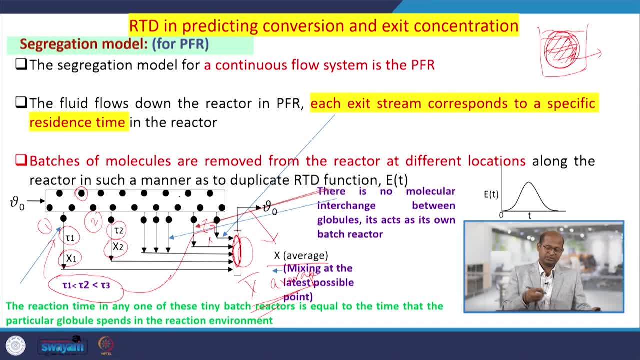 individual. So we can consider as a in the inside of the plug 4 reactors, individual globules. we can consider or acts as a individuals batch reactors where the molecules does not interchange with other globules. So therefore, here the conversion inside of the reactor should be or inside of the globules. 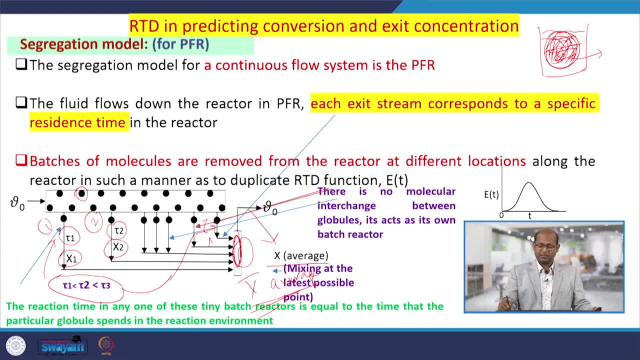 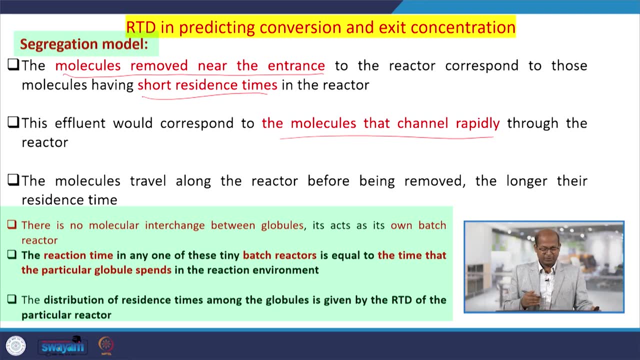 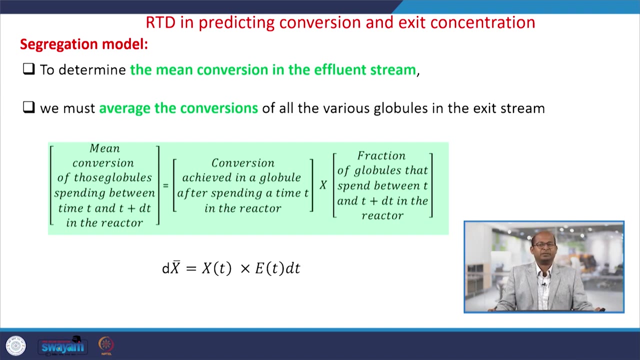 should be same anywhere but one globules to other globules. the conversion concentration should be different. So these globules and these globules, two different globules having different concentration, different conversions. So now, based on these is assumptions and based on that, If we, from the exit outlet, we want to measure the concentrations and if you want to find 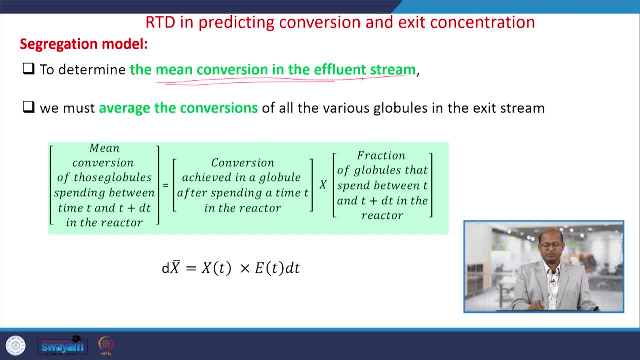 the conversions. so then, average concentration of the effluent stream or mean conversions, we can get The average conversion for all the globules. that is the exit stream that we will get. so this, So here, dX bar, that is the mean conversion's of those globules spending between time t. 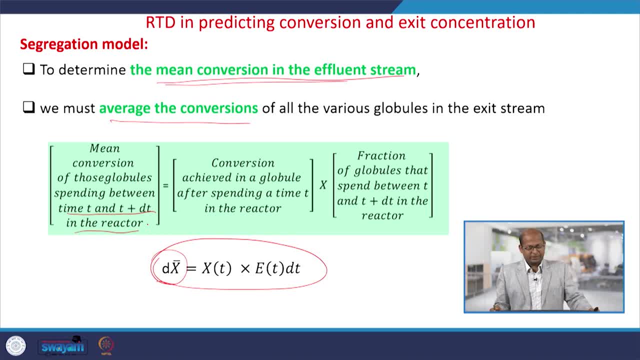 T and T plus DT in the reactors and then conversions achieved, each globules after spending time T inside of the reactors. So this corresponds the individual globules we have considered and this is the XT Here: individual globules having the conversion that is XT, individual. 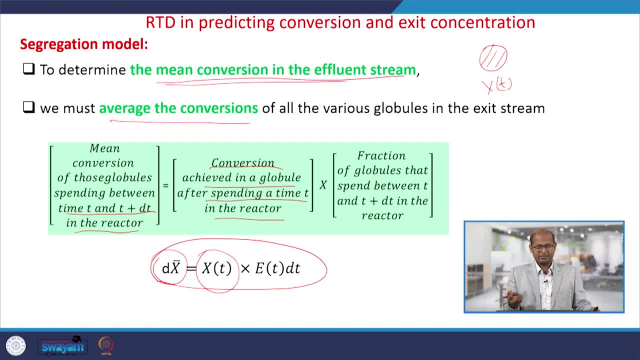 globules. we are considering a single batch reactor and if the reaction is, let us say, first order reaction, and if we know the reactions rate, constant for these reactions, and so then the average or these conversions, individual globules, we can find out, and then within that, the fraction of materials living, that fraction of globules that spend between T and T plus. 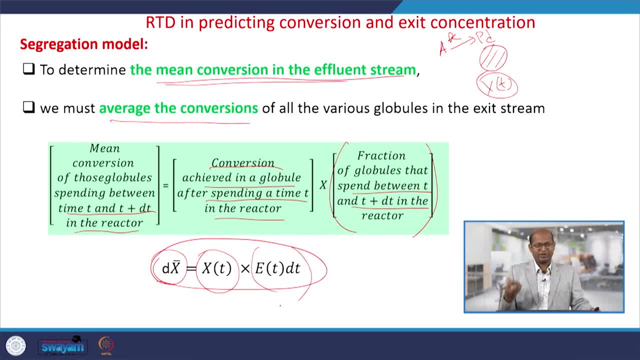 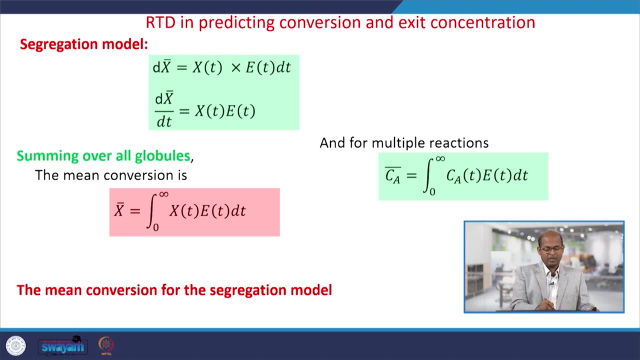 DT, if we know, So that residence time or fraction of molecules, if we know, and the conversions, if we know, then average conversions we can find out. This is the from the segregations model. this equation is the key equation to find out, So we can find the average conversions. So now, if we write the equations this way and 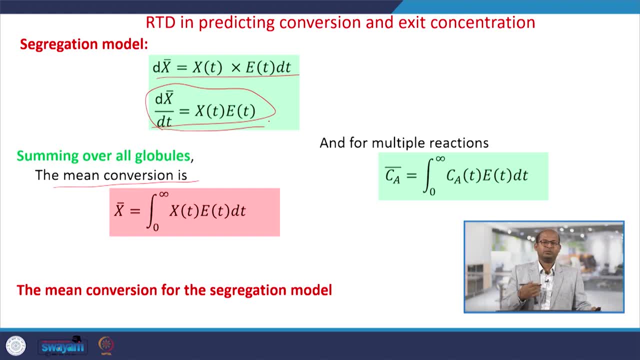 integrates means: since there are n number of globules, so many globules are there. So if we integrate this equation, these equations, and then in the left hand sides, after integration 0 to infinite, we get X bar. that is the average conversions that we are getting from the exit. 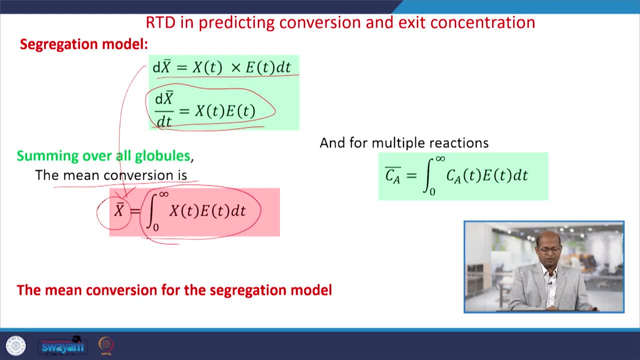 point of the reactors And in the right hand side. so what are that? components are present, that is, the conversions from individual globules and that is the residence time distribution. function for that? components or is globules? So therefore, for overall systems conversions, if you want to know, or 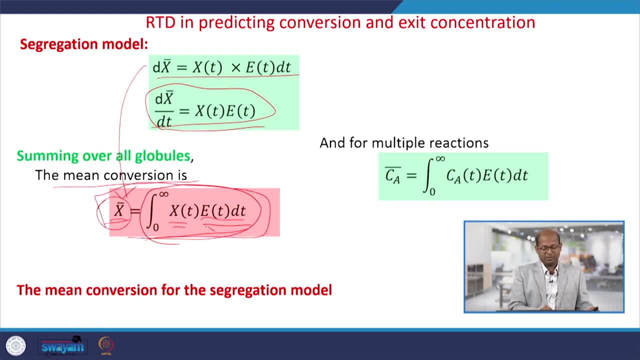 that is the mean conversions. these equations you have to find out and then, depending upon the reactors- either it is FlaK 4 reactors or CSTR reactors- we have to put the residence time, distribution functions and then average conversions We can find out using this particular models, Similarly the average concentrations also. 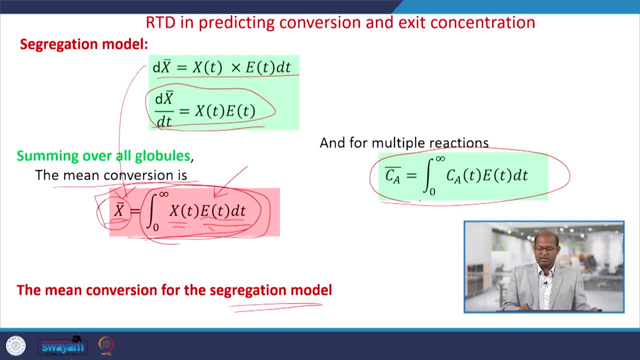 we can find out using these equations. that equation is similar here: C A, bar is the average concentrations and C? A is the individual globule concentrations and E t, d, t, that is the residence time distribution. C t is the residence time distribution for that particular. if we sum: 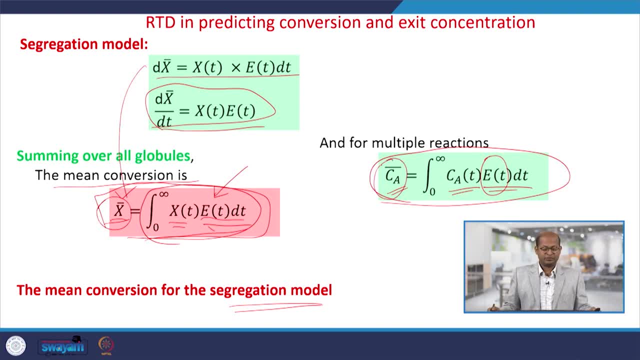 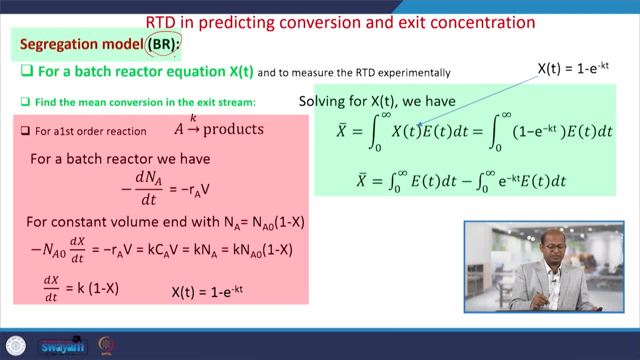 up from 0 to infinite time. So then average concentrations we can get from the segregations models. So once we know the segregations models, so now consider a batch reactors if you want to find out the average concentrations or average conversions. So then this is let. 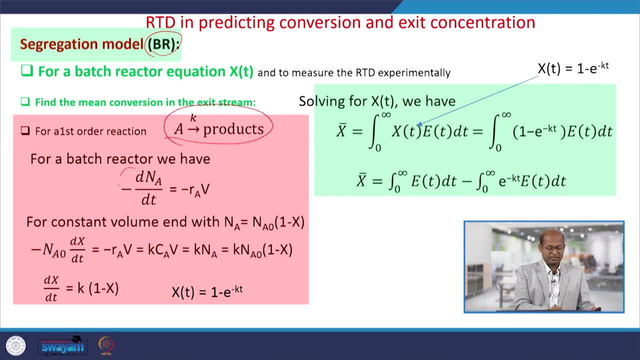 us say reaction, first order, reaction that I said. So batch reactors design equations. or minus d, n, a by d, t equals to minus r, a v, that we know. and n equals to n or a, not into 1 minus x, that we know, for that concentration on moles, that way changes finals. this is initial. 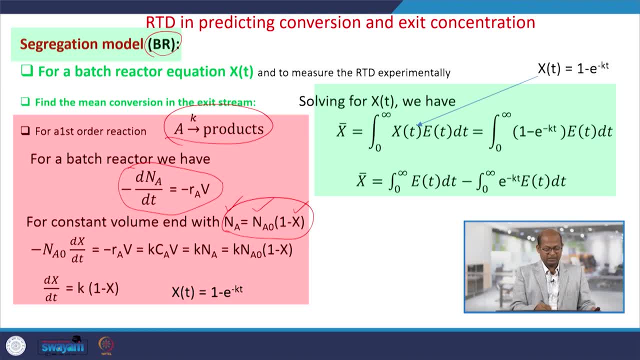 this is conversions. So if we substitute that in that equations and after this differential equations, simplifications, we can get this, and after integrations of these equations we can get X, t equals to 1 minus e, to the power minus k into t. that is, the conversions inside of a batch reactors. 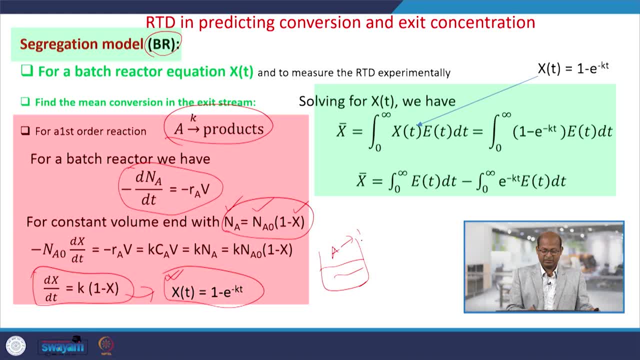 Let us say we have a batch reactor here we are conducting these reactions. So here are the conversions, what would be the conversions? that equations we can write 1 minus e to the power minus k into t. So here, if we know reactions rate, constant and time, so then 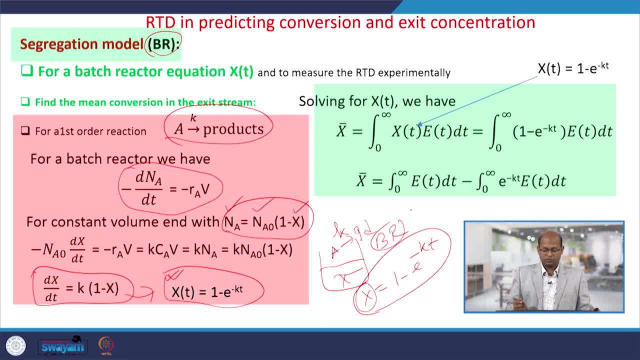 what would be the conversions for this particular batch reactors? we know. So in segregations model, each globules we consider a batch reactors, so therefore each globules must have conversions, this or this. So the conversions we are substituting here, considering each globules, what are the molecules spends? this is a batch reactors and if it, 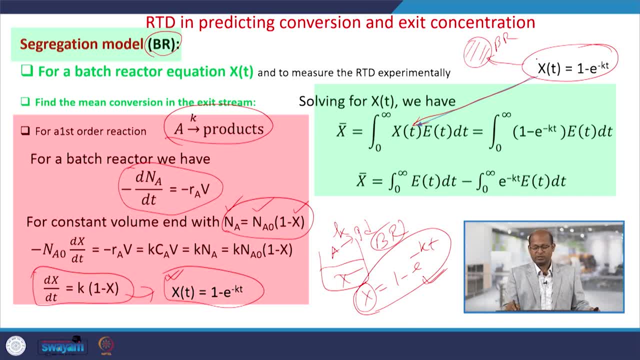 is batch reactors For one globules, the conversion is this: so, like that, a number of globules are present. So then we can substitute here and these equations we can simplify, and then we can get these equations- For this is the general equations- to find out the average conversions for the molecule. 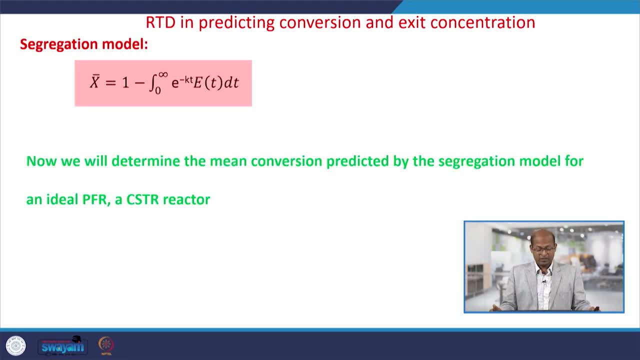 spending and considering the segregation models. So this is the final equations, or equations we can get. Now we have to determine the conversions by considering a ideal plaque 4 reactors or ideal C-H-T-A reactors. This is the general equations we have find out by using segregation models. 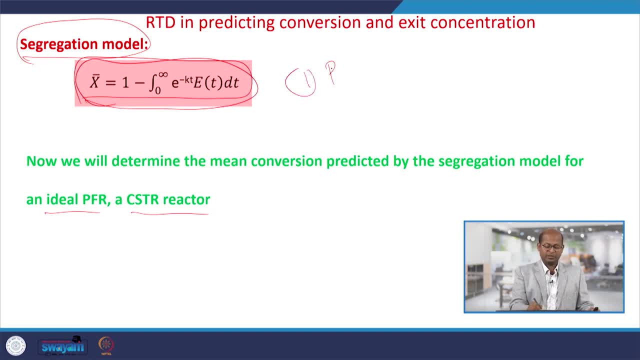 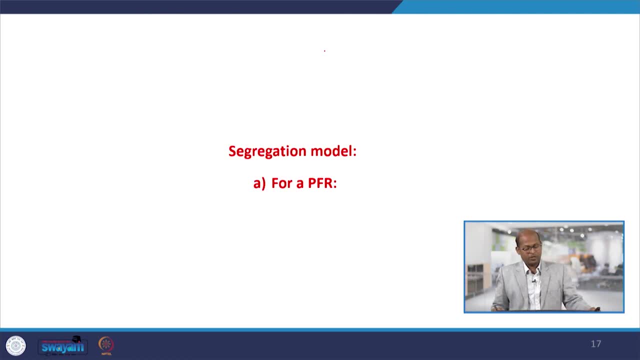 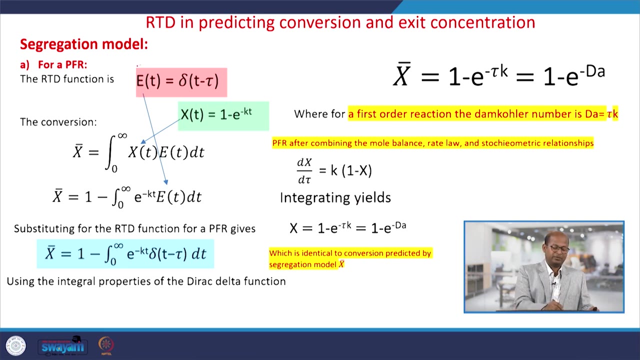 So now these models we can implement either a PFR or we can use a C-H-T-A reactors. So one by one, we will discuss. So first consider a plaque 4 reactors: implementing the segregation models in a plaque 4 reactors. So ideal plaque 4 reactors. 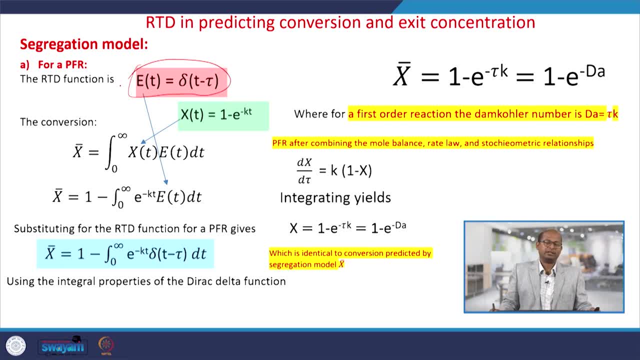 The ideal plaque 4 reactors residence time distribution functions is E. T equals to delta T minus tau, So that we have discussed in your previous class. So therefore E- T- we can consider this and here we are considering reactions- is a first order reactions. n equals to 1, that is a first order reactions. 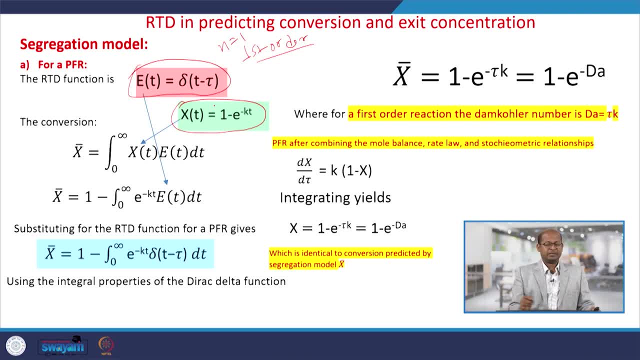 So then it is equals to delta T minus tau, and X T equals to 1 minus T, to the power minus K T. both we are substituting in these equations. So then we can get this. So now we have to do more reads. 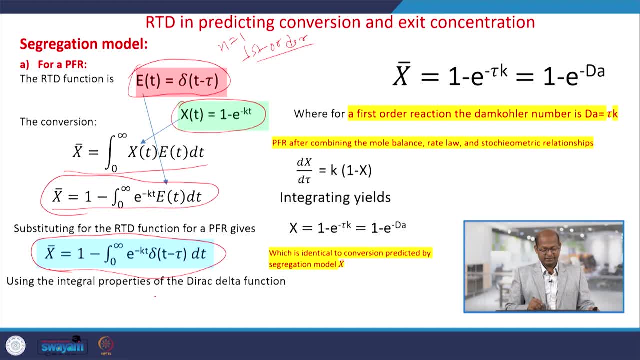 Next, Next, Next, Next, Next, Next, Next or after substitution, we can get this. So this is the now, this equations, this component part. if we consider so, then it would be like this: So x bar equals to 1 minus this part. 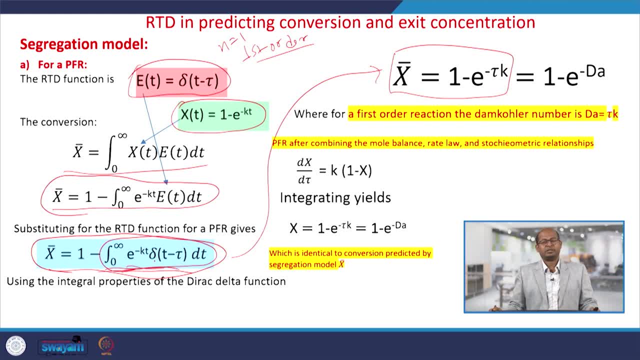 actually integration: 0 to infinite. e to the power minus kT, delta T minus tau dt, So that would be e to the power minus tau k. So this is equals to, or 1 minus e to the power minus dA, or dA equal to Damkohle-Namka that we have discussed in our previous class, when 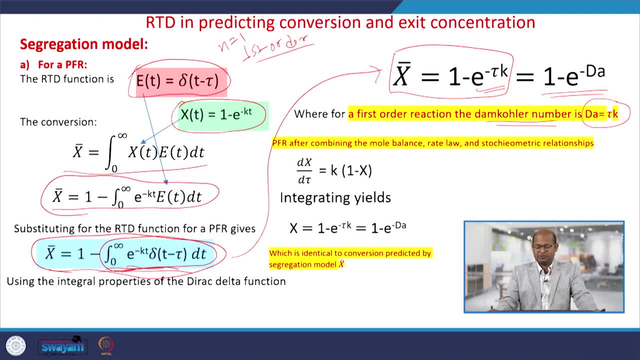 we have studied the residence time or space times. on that times we have discussed what is the Damkohle number for first order reactions. dA equals to tau k, or this way, or either this way we can express So from the segregation models. the average conversions, that is equals: 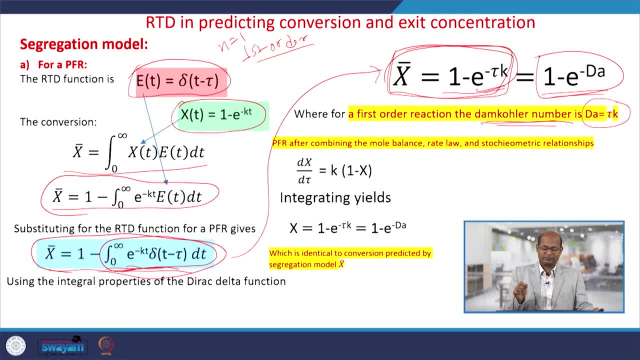 to 1 minus e, to the power minus tau k. So this is for PFR reactors. So that way means we have developed from the segregation models. So if we do not have segregation models from the flag flow reactors also, this type of equations also we have developed earlier from this equations if we integrate. So this: 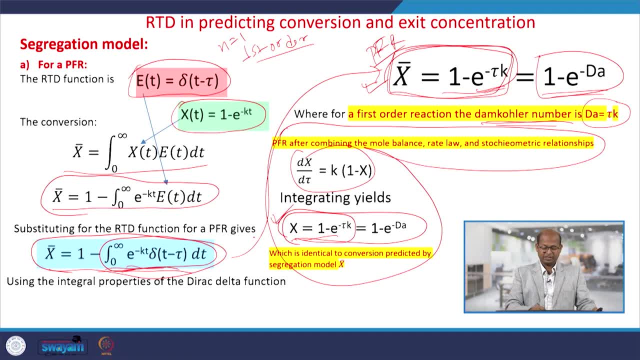 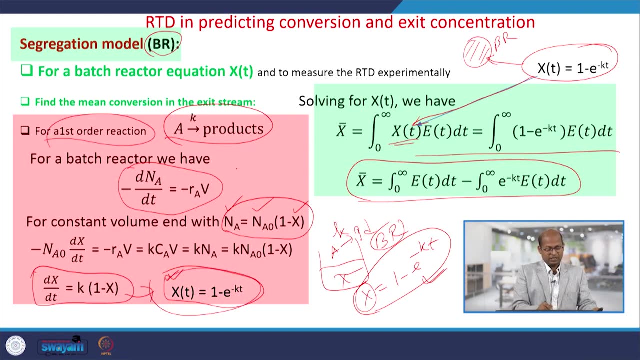 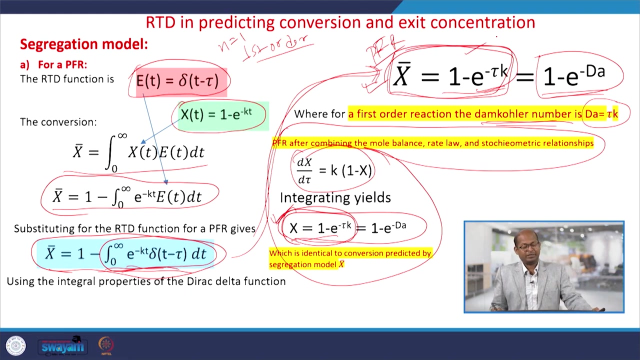 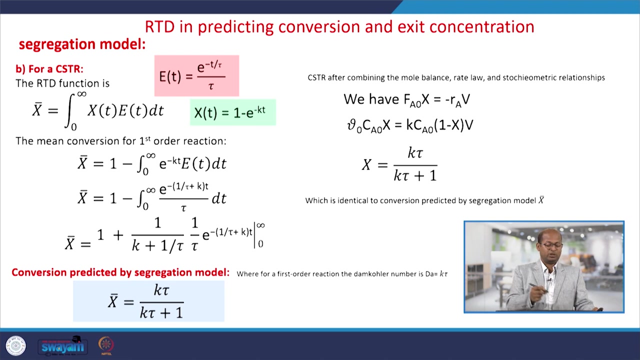 way we can get this. So both the equations you can notice. So from the segregation model we are getting these equations. So again, the first section regarding the Tesla blend is: what is thatestä? This is the water molecular exchange. adults mix them by these two vectors and apply the segregations. 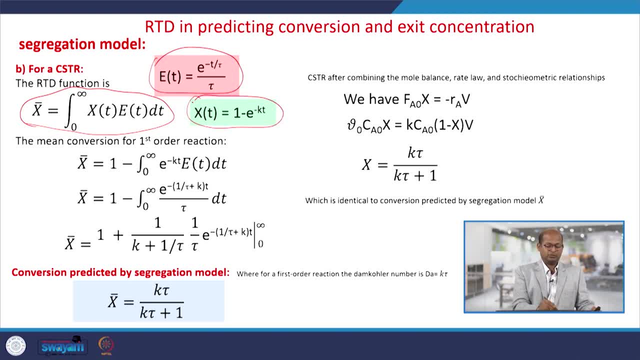 model. So this is the general equation. average conversion that we are getting from the exit point of the reactor is these: And residence time and distribution functions. for a C package ésc connection system. Reactor C is this: and X, t equals to 1 minus e to the power minus. 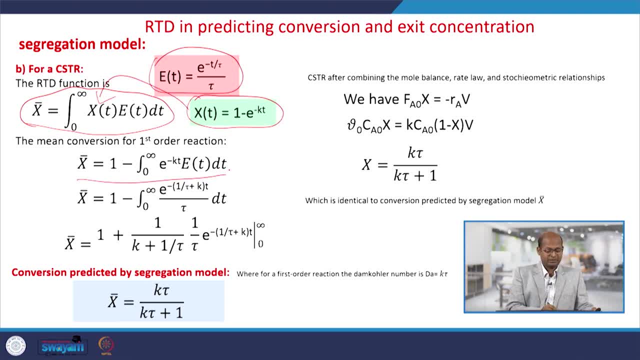 k, t that we have received from batch reactor data analysis. So now this two, 1 by 1. if have to substitute, here we can get it, and then, after simplifications, we are substituting Et. So then, if we simplify these equations then it would be like this: So x bar equals. 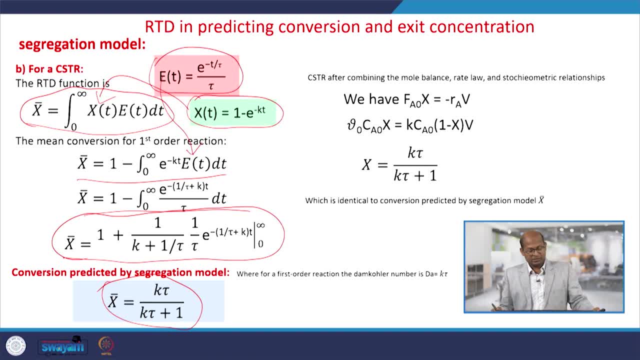 to tau k by 1 plus tau k. So that is the predicted conversions or average conversions. and from the Siester mole valence equations also similar equations we have developed, so both are identical. So means, by considering segregation models, the equations we are getting 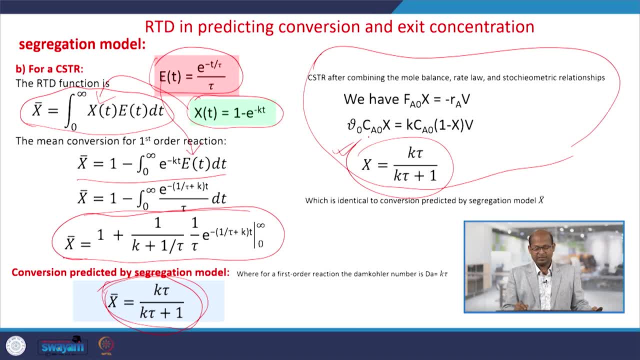 to find the average conversions and by considering these reactors models for a Siester reactor from the design equation this type of equations are also. we are getting So both are the equations are similar. So from the model equations we can use these equations to find. 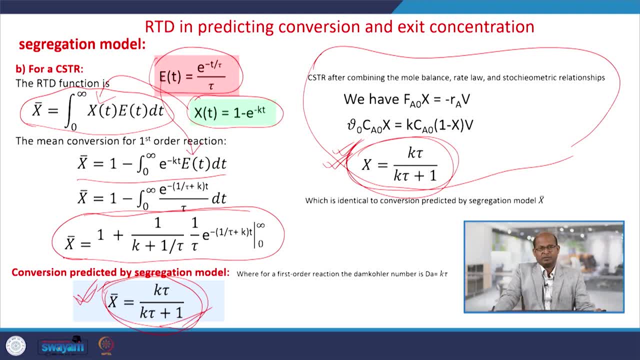 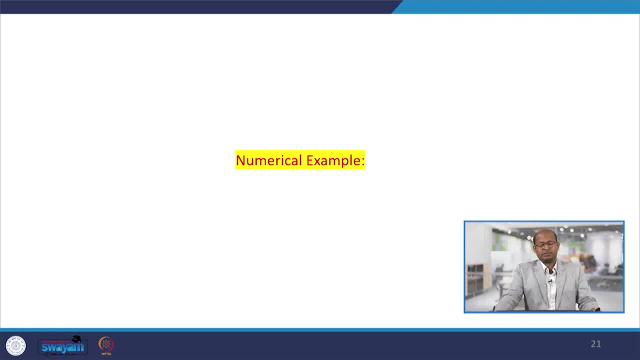 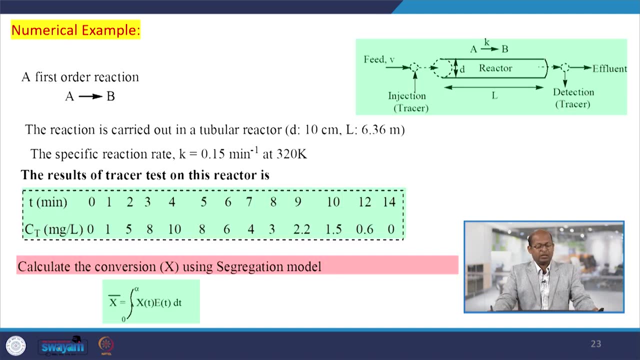 the average conversions for this particular model. So this is a reactor, by considering the residence time distribution functions. So now one numerical problems or examples we will discuss, considering the segregations models and considering RTD distribution functions, how we can find the average conversions. 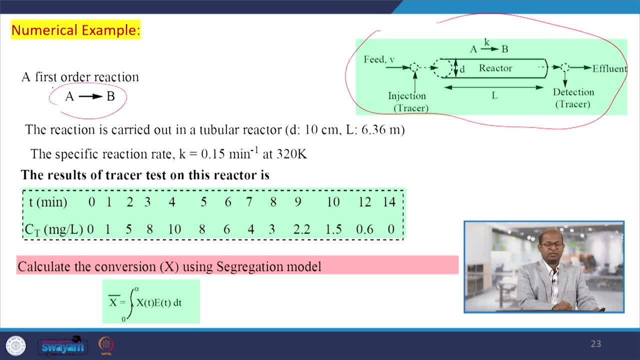 Let us say this is a reactors. let us say here we are considering these reactions and in this particular reactions, rate constant that is given at 320 Kelvin is given and see here if we conduct a TREASURE test or RTD study or TREASURE test, TREASURE test: if we consider 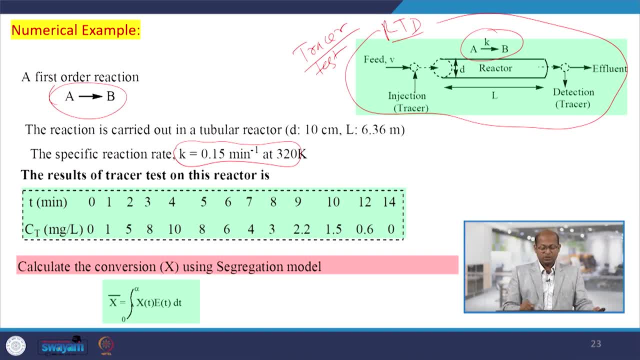 for this particular reactors, so without conducting reactions. So then the pulse TREASURE injection. so here the TREASURE concentrations at different CT, TREASURE concentrations at different times. we can find out. So this table is given. So this is the residence time distribution. 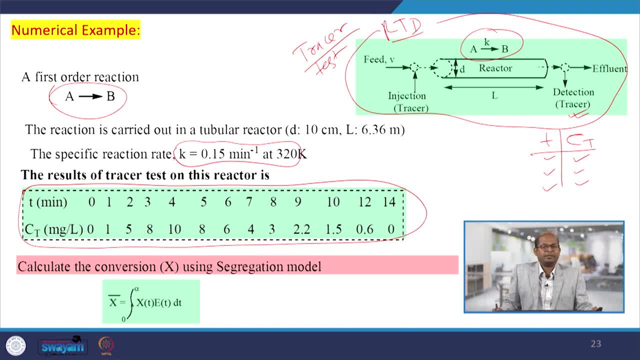 functions and TREASURE test results is given. So the TREASURE test results is given In. So with that treasure test, how we can find out the conversions if we conduct these reactions here. So number 1 is the treasure test. 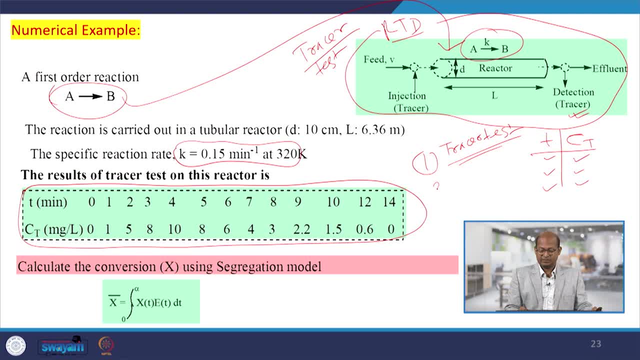 So, considering this treasure test, we can predict the average conversions for these reactions. Here reactions rate constant is given, We are not conducting these reactions here. Similarly, we can predict by whatever that we have the treasure test and with the help of the treasure test we can find out the average conversions by considering the segregations. 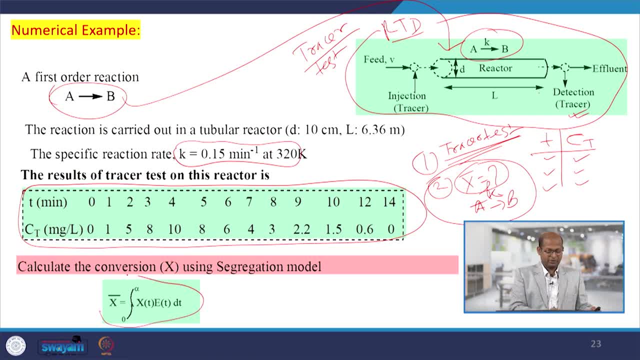 model. So now in the segregations models the average conversions equation is this: X bar equals to 0, to infinite, Xt Et. these equations we know that we have developed for segregations models, So we have treasure test experimental data. 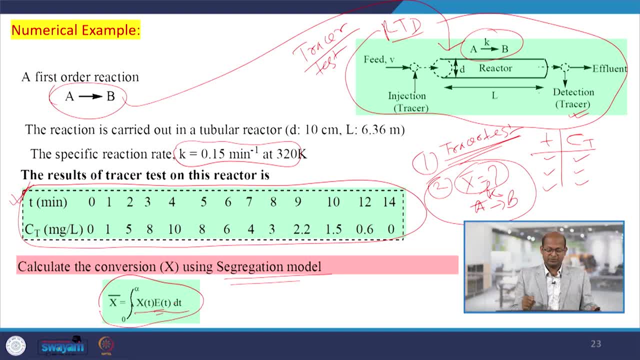 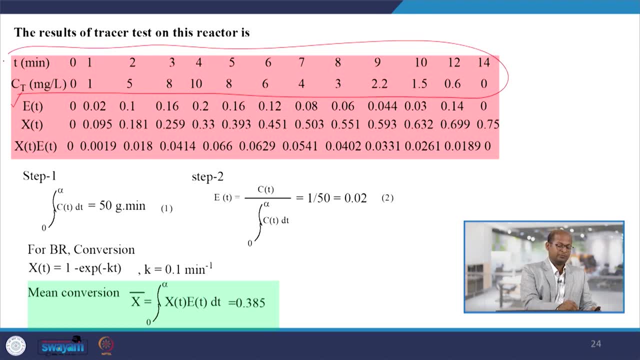 So now what we have to find out, Et. So this is the residence time distribution for these reactors we have to find out. So first we have to find out from the. this is the data is given from the or collected from the treasure test experiment. 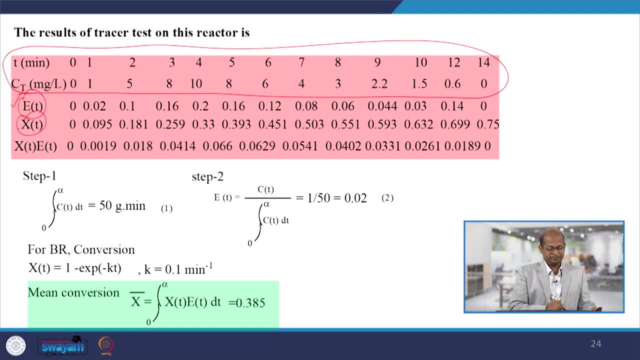 Then we can find out Et, We can find out Xt, Then Xt into Et, we can find out Xt. This was used for to find the Xt. So here we know K and T, So Xt we know. So now these are the components we developed, or these tables we have developed. 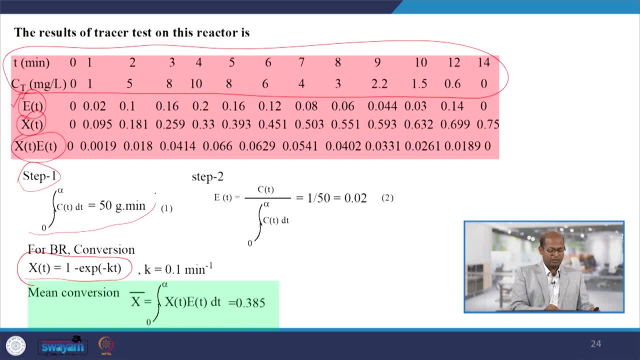 So now, step 1 means to develop these tables. we need this, we need Et. Once we know Et and Ct from Ct we know means first we have to find out Ct, C curves, then E curves are Et. So this Et has developed using this and Ct at this point means this: we have to implement. 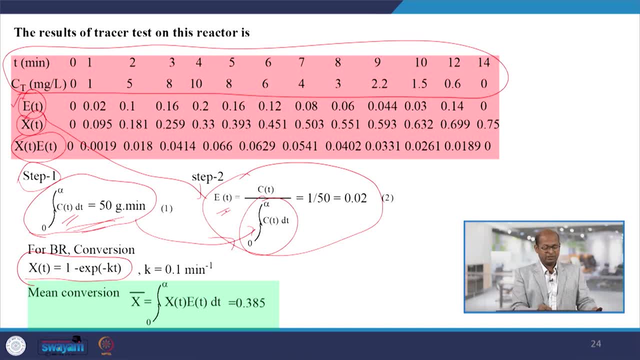 here apply here Then. So we can get only Et. So how a time and concentrations, the data we have from there, how we can find out Et, So that is given by step 1 and step 2.. Then Xt also, we can find out that rate constant for this particular reactions is given. 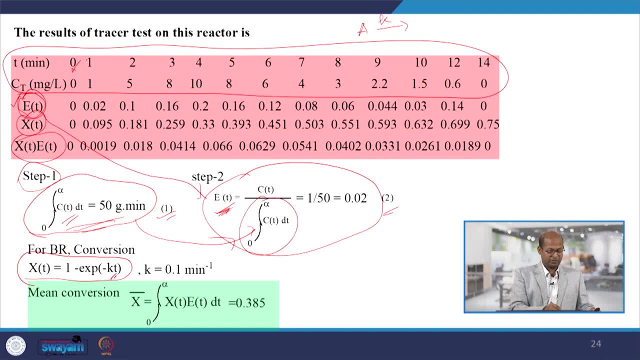 That is, K value is known. So then at time is known, at this particular times we can put Xt value. we can find out, And then this we can Xt into Et We can, So we can find out from this tables we can get. 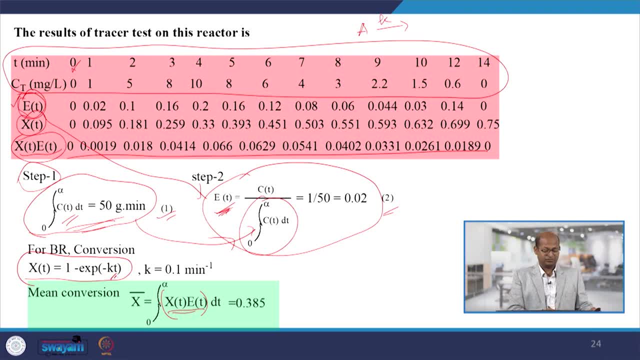 So now, if we do integrate 0 to 14 minutes, So then this value after integrations that would get this. So by using Simpson's one third rules that we have discussed already, Simpson's one third rules that have to implement or other rules are available to integrate. 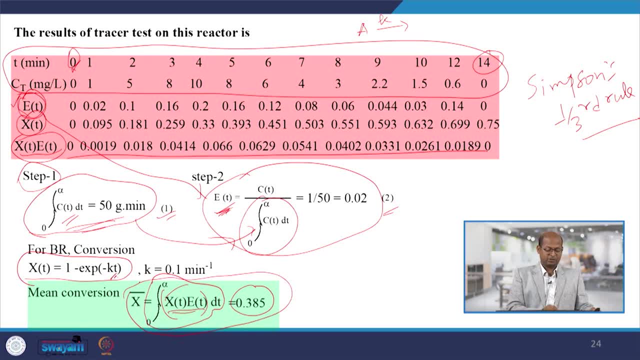 So we can find out, Solve this integration, so that we have discussed in our previous class along the back that class we have taken. So there we have discussed this. So therefore from here we can find the mean conversions for this. reactions means we have. 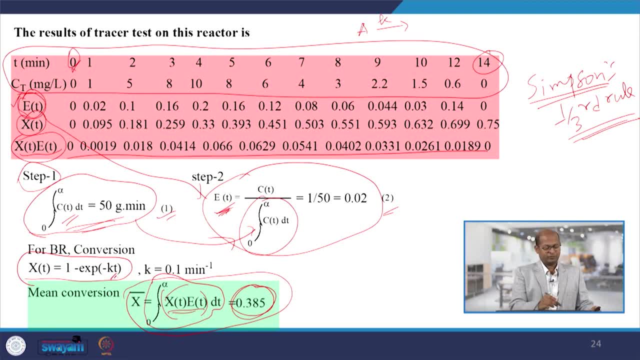 conducted only tracer test. This is the tracer test results. this is the tracer test results. So CT. So with the help of tracer test and reactions rate constant. so that is the things are known. using this equations means segregations, model equations- we can predict what would be the 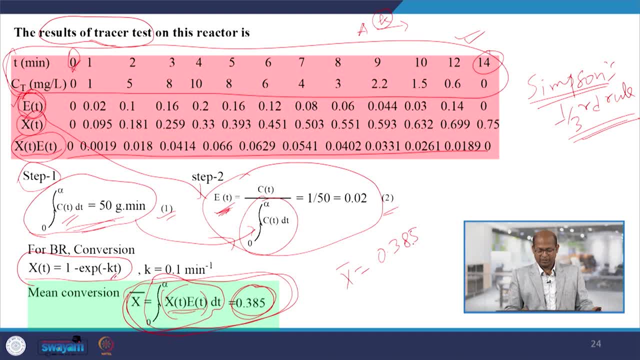 average conversions. that is 38.5 means 38.5 percent conversions we can get. So if we conduct the reactions in a that particular reactors where that tracer test was conducted And this data was obtained, then if we use the segregations models, so then we can get. 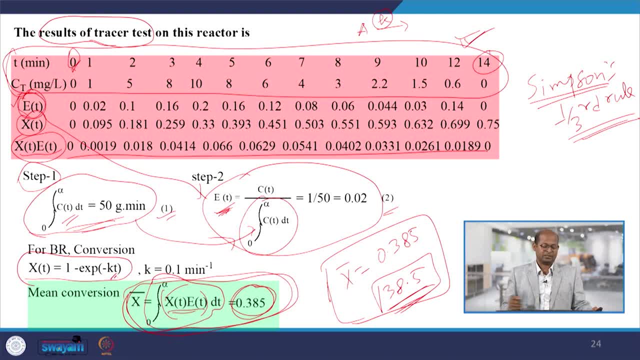 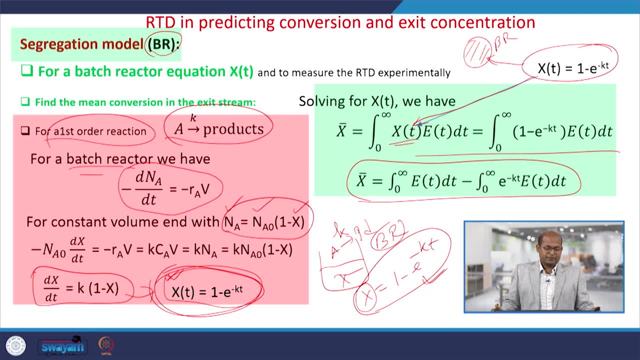 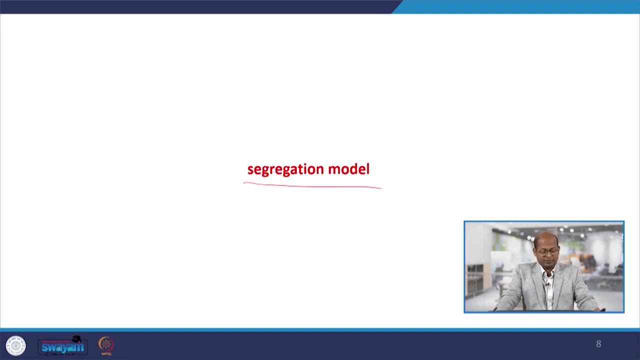 38.5 percent conversions for this reaction. So this is the take home means. what are the things we have studied? So first we have discussed about the different type of mixing and what are the different models are available and based on that we have considered segregations model and segregations. 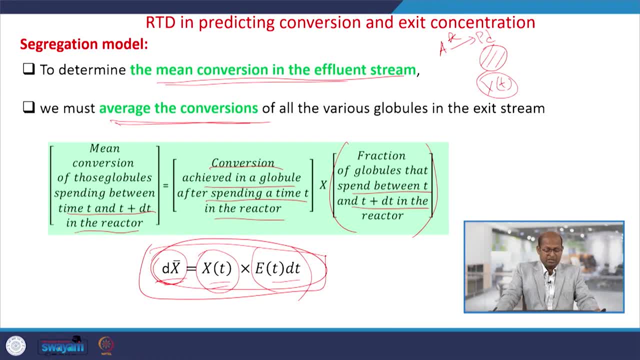 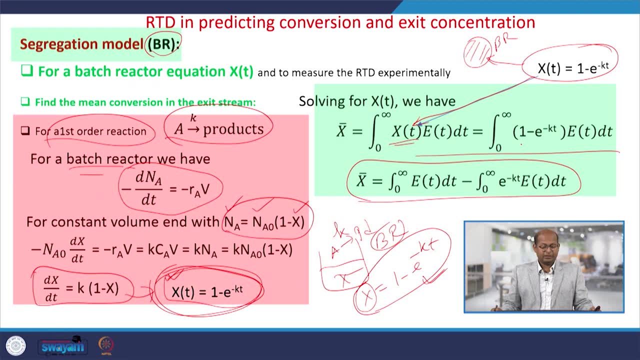 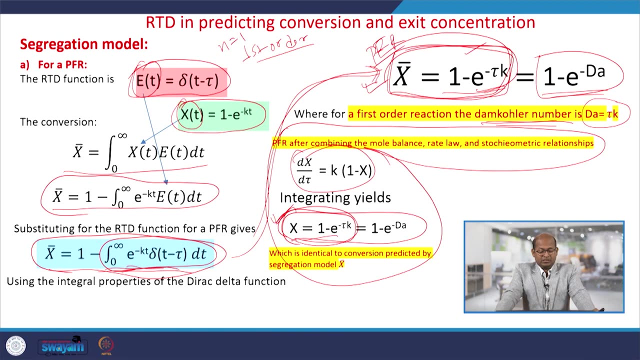 models. So we have discussed and we have derived this equations and then mean conversions and mean concentrations, equations we have developed and then so we have applied that to in a CSTR reactors and plaque 4 reactors and that final equations we have developed and considering.